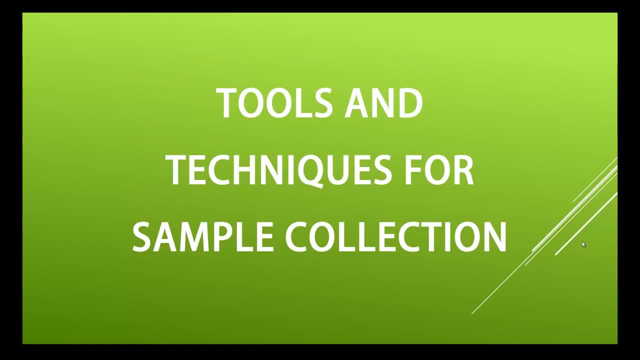 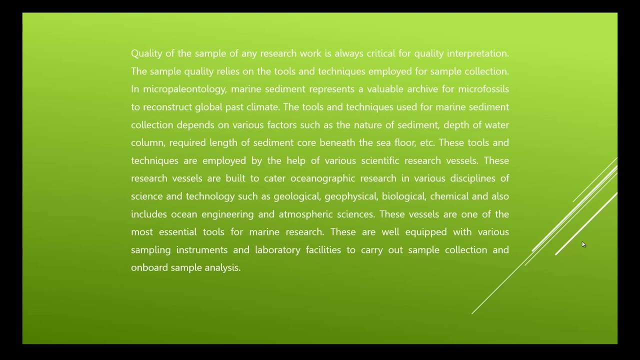 employed for sample collection. Now let us see what are the various techniques, tools and techniques used for sample collection in micropalentology. To carry out deep sea marine sediment sample collection, various scientific research vessels are used. These research vessels are one of the most essential. 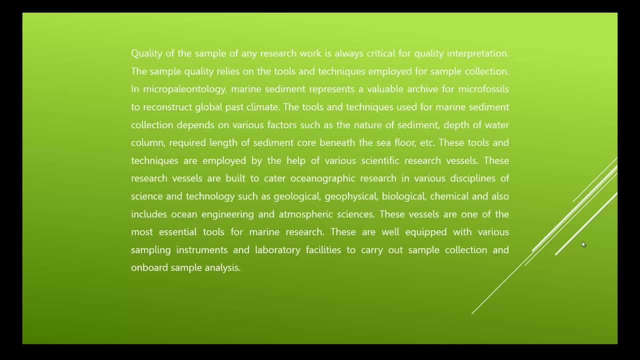 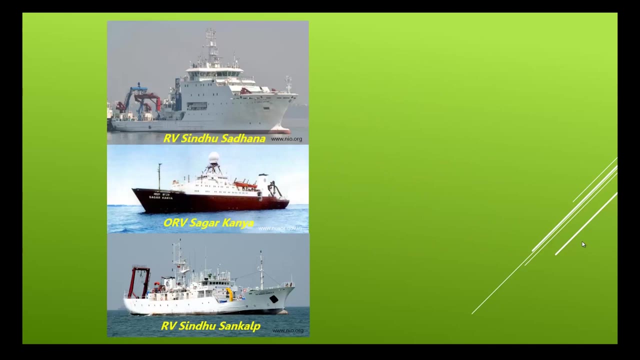 tools for marine research. These are well equipped with various sampling instruments and laboratory facilities to carry out various sample collections and on-board sample analysis. In India there are many oceanic research vessels acquired by various government research organizations, For example, RV Sindhu Sadhana, RV Sindhu Sankal, ORV Sagar Kanya, RV. 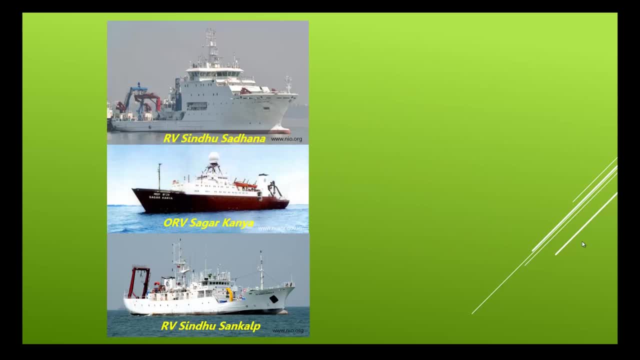 Samudra Ratnakar, ORV Sagar Nidhi and Sagar Manjusha are the major ones Among them. the research vessels RV Sindhu Sadhana and RV Sindhu Sankal are a multidisciplinary 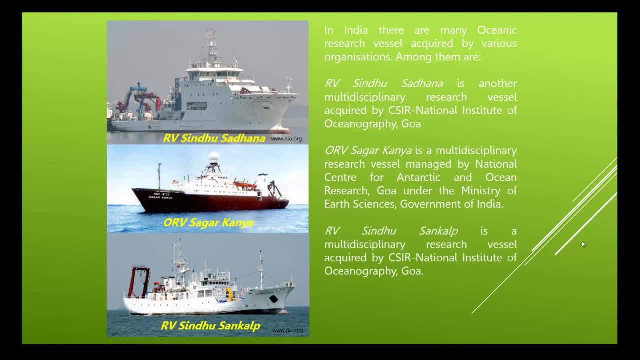 research vessel acquired by CSIR. Likewise, ORV Sagar Kanya is also a multidisciplinary research vessel managed by National Center for Antarctic and Ocean Research under the Ministry of Earth Sciences Government of India. RV Samudra. 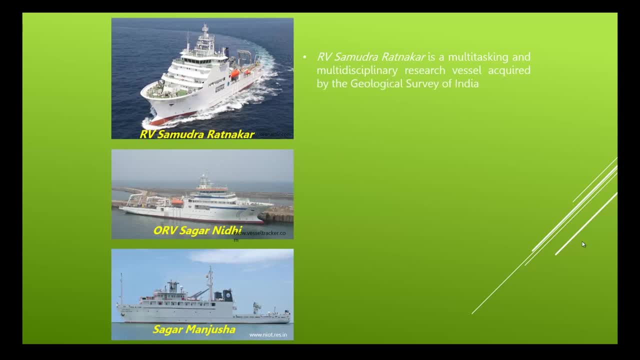 Ratnakar is a multi-tasking and multidisciplinary research vessel acquired by Geological Survey of India. ORV Sagar Nidhi is an ice-class research vessel. RV Sagar Nidhi is an ice-class research vessel. RV Sagar Nidhi is a multi-tasking and multidisciplinary research vessel acquired 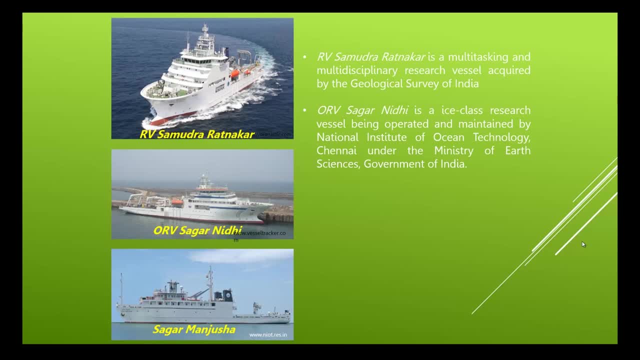 by CSIR under the Ministry of Earth Sciences Government of India. All these research vessels are capable of navigating through the ice-class. ISE class means it can navigate through the ice sea. This research vessel is operated and maintained by the National Institute of Ocean Technology Chennai under the Ministry. 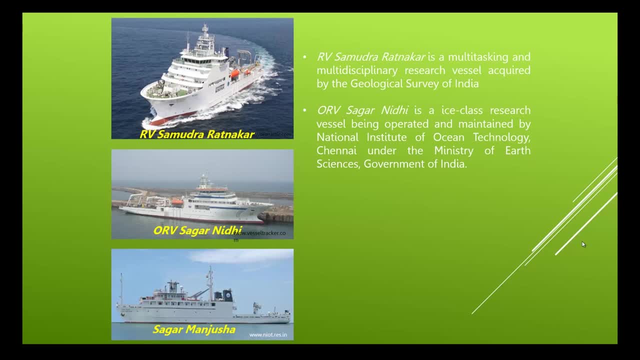 of Earth Sciences Government of India. The next one is Sagar Manjusha. It is again a multidisciplinary research vessel acquired by the National Institute of Ocean Technology Chennai under the Ministry of Earth Sciences Government of India. So all these research. 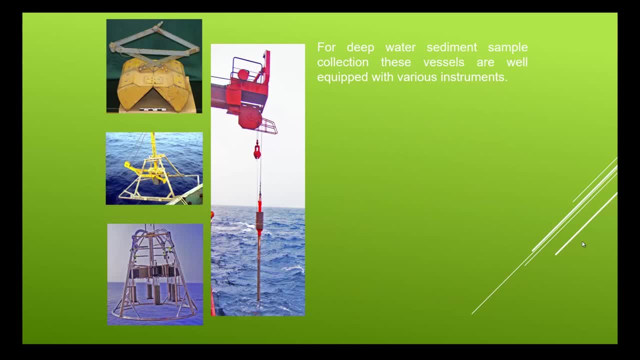 vessels are capable of deep-sea sediment sample collection from the unconsolidated upper part of the seabed. For deep-water sediment sample collection, these vessels are well-equipped with various sampling instruments. Again, there are several types of deep-water sediment sampling instruments. 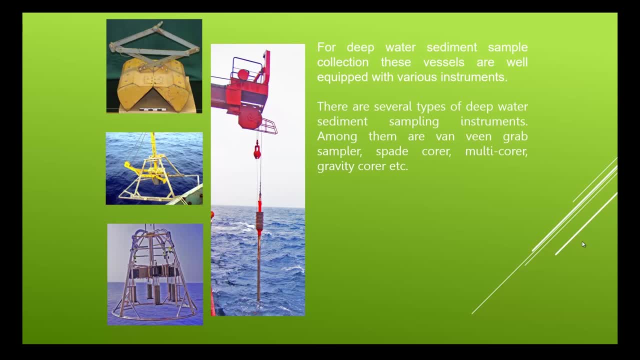 Among them are wind-wind graph sampler, spade corer, multiple corer, gravity corer, etc. Depending upon the requirement of sample, at different water depth and length of the sediment core beneath the seafloor these instruments are deployed. 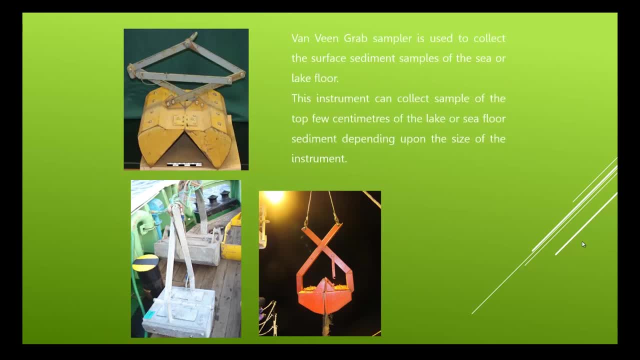 For surface sediment sample collection of sea or lake floor graph sampler is used. This is also known as wind-wind graph sampler. This instrument can collect sample up to the top few centimeters of the lake or sea sediment, depending upon the size of the instrument. 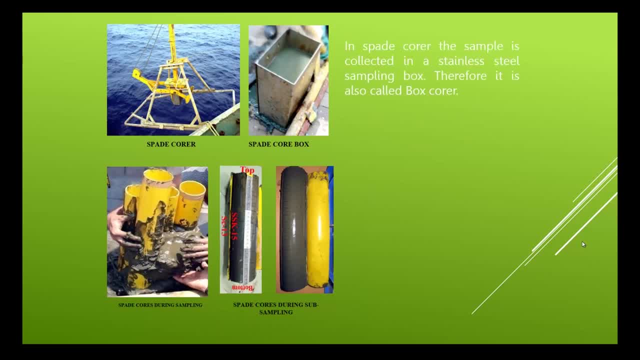 Now come to spade corer. In this corer, the sample is collected in a stainless steel sampling box. Therefore it is also known as box corer. It comes with various sizes, based on their different length, breadth and height of the. 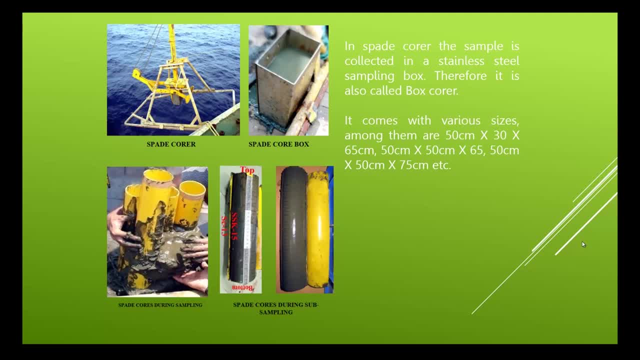 box, For example, 50, 30,, 65 cm, 50, 50, 65 cm, 50, 50,, 75 cm, etc. So in this device we can collect sample of the top two. 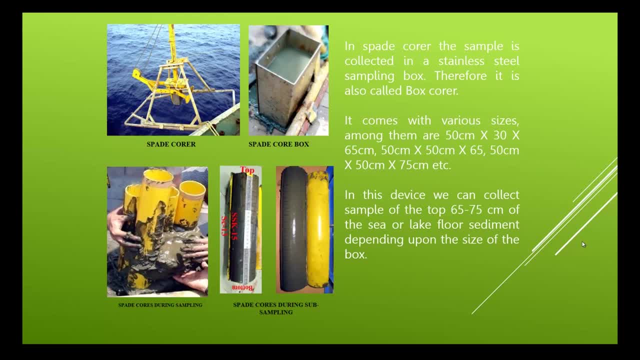 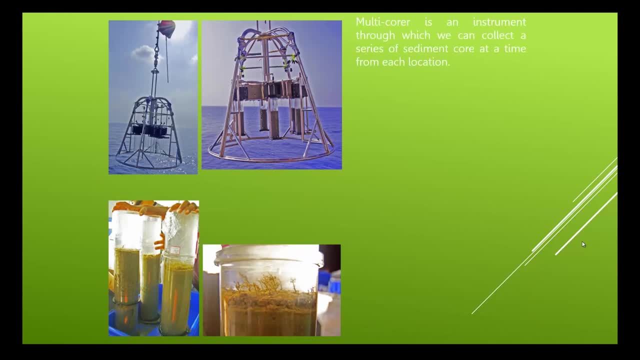 So we can collect sample of 65 to 75 cm of the seabed, depending upon the size of the box. Now come to multi-corer. Multi-corer is an instrument through which we can collect a series of sediment cores, that is, a maximum of eight cores at a time from a given location. 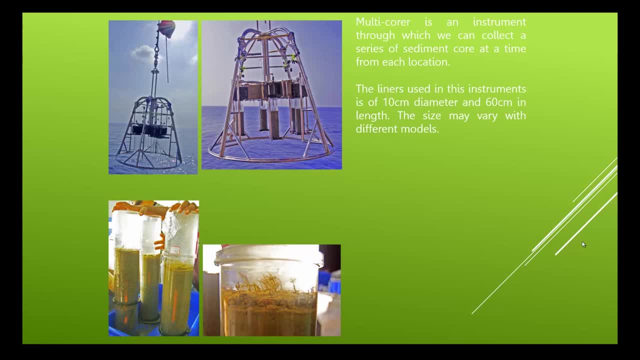 The liners used in this instrument are made up of acrylic material to avoid any contamination caused by metal body to the sediments. The standard size of the liners are of 10 cm in diameter and 60 cm in length. The size may vary with different models. 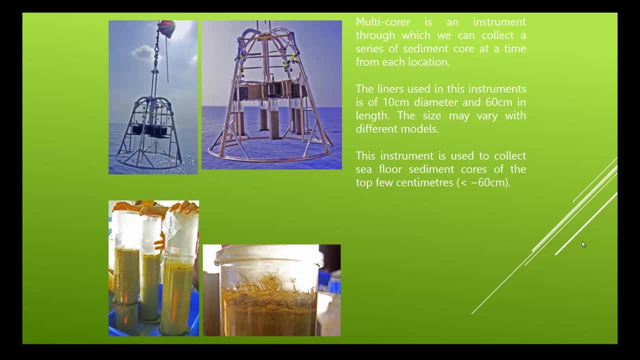 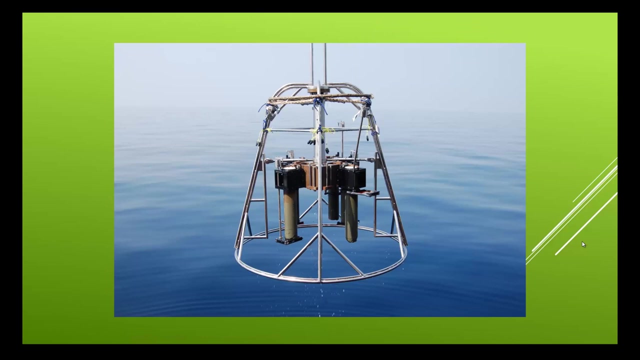 This instrument is used to collect seabed sediment cores of the top nearly 60 cm of the seabed. This device is very unique in collecting fully undisturbed core sediment samples along with the overlying few centimeters of the bottom one. We can collect this water for various bottom water studies. 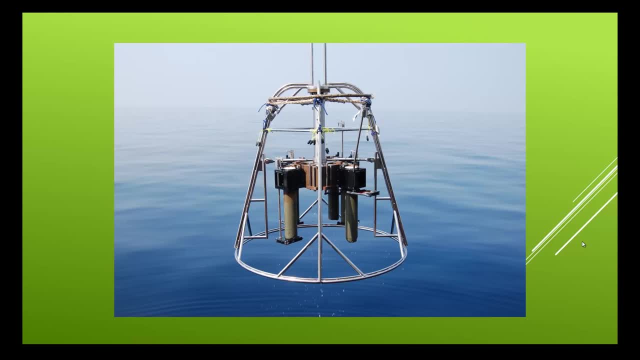 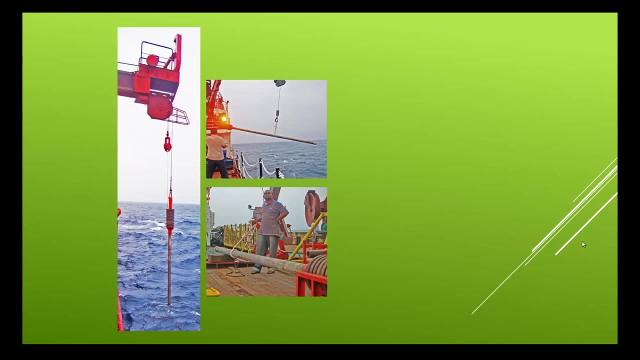 In this picture we can see the seagrass inside the liners, and that gives the evidence of totally undisturbed seafloor. The next instrument is gravity corer. This instrument uses the pull of gravity to penetrate through the seafloor, sediment and 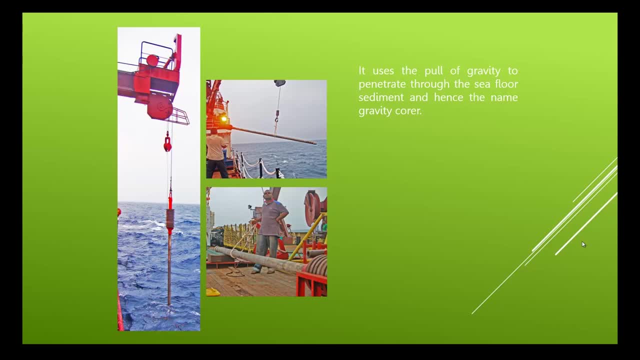 hence it is called gravity corer. The standard length of the corer is 10 cm. The length of the corer is 10 cm. The length of the corer is 10 cm. The top diameter of the corer is 6 m and the diameter is 15 cm. 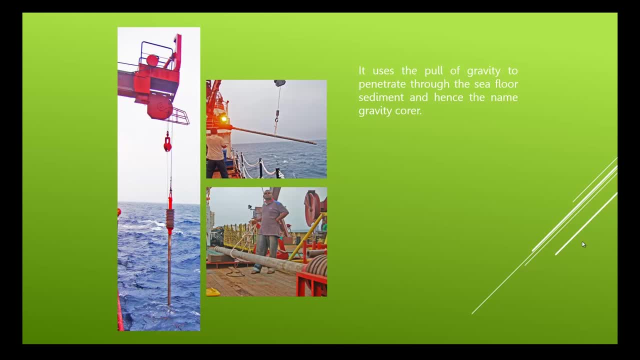 The size may vary with different models. This instrument is used to collect seabed sediment cores up to the top six meter of the seabed. All these sampling instruments are restricted to the upper few meters of the seabed In order to assess, for a longer time period in geological past, longer sediment cores. 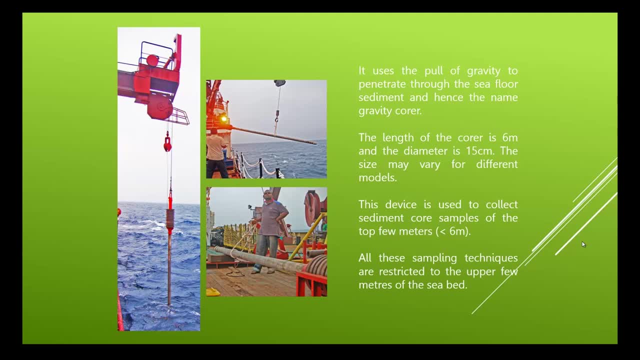 are required extending much deeper beneath the sea floor. For this purpose, research vessels having drilling capability are used to execute the task. Among them are JOIDUS, Resolution and CHIQU. These are the deep sea drilling research vessels capable of retrieving sediment pores, extending 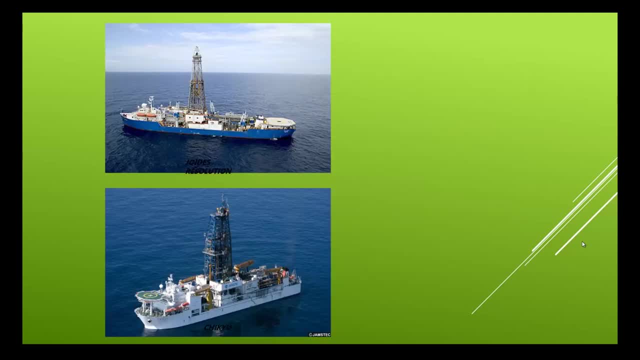 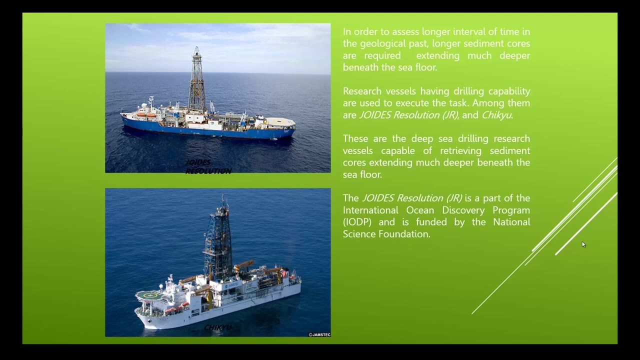 much deeper beneath the sea floor. The drilling ship JOIDUS Resolution is a part of the International Ocean Discovery Program, or IOTP, and is funded by the National Science Foundation. Similarly, CHIQU is designed by the Japanese government for international scientific drilling operations. This drill ship can drill up to 7000 meters below. 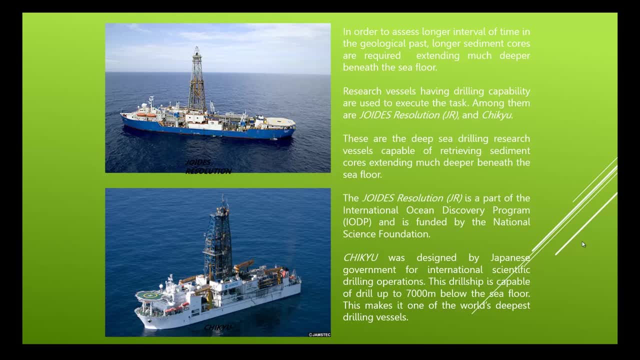 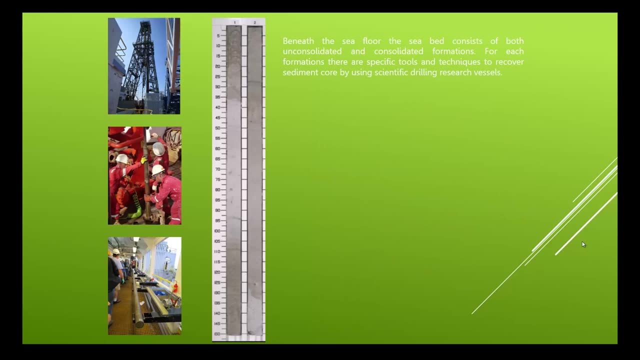 the sea floor. This makes it one of the world's deepest drilling vessels. Beneath the sea floor, the seabed consists of both unconsolidated and consolidated formations. For each formation, there are specific coring techniques to recover sediment cores. Among these coring techniques, the first one is Advanced Piston. 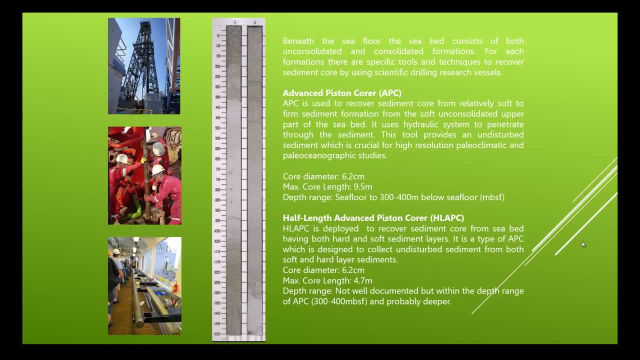 Corer or APC. APC is used to recover sediment cores from relatively soft to firm sediment formations of the soft, unconsolidated upper part of the seabed. It uses a hydraulic system to penetrate through the sediment. This tool provides an undisturbed sediment, which is crucial for high 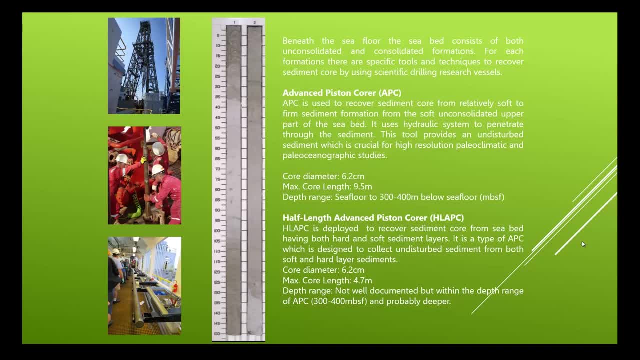 resolution: paleoclimatic and paleoceanographic studies. In this coring technique, each core comes with a maximum length of 9.5 meters with a diameter of 6.2 centimeters. The depth range of this coring technique is from sea floor to 300 to 400 meters below sea floor. The second coring technique is 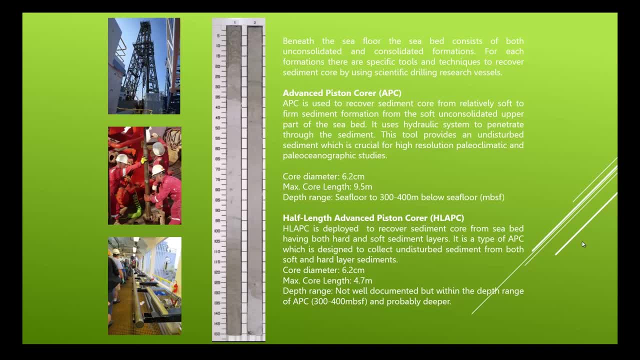 Advanced Piston Corer, or Half-Length APC. This half-length APC is deployed to recover sediment core of seabed, having both hard and soft sediment formations. It is a type of APC which is designed to collect undisturbed sediment from both soft and hard layer sediments. Here each core comes. 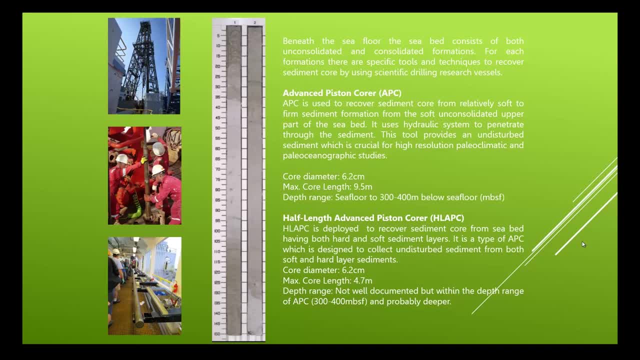 with a maximum length of 4.7 meters with a diameter of 6.2 centimeters. The depth range of this coring technique is not well documented, but within the depth range of APC depth, that is, 300 to 400 meters below the sea floor, or probably much deeper. The third one is Rotary Core Barrel. 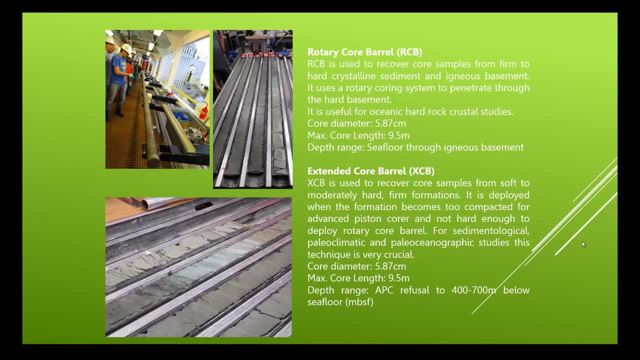 or RCB. RCB is used to recover core samples from firm to hard crystalline sediment and igneous basement. It uses a rotary coring system to penetrate through the hard basement. It is useful for the forming of the core in the core trouvé. The fourth one is Oceanic Hard rock crystal studies. 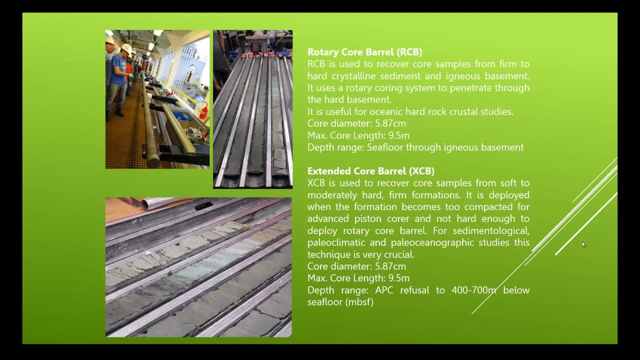 In this coring technique, each core comes with a maximum length of 9.5 meter with a diameter of 5.87 centimeter. The depth range for this coring technique is sea floor through igneous basement. The fourth coring technique is Extended Core Barrel, or XCB. XCB is used to recover core samples from 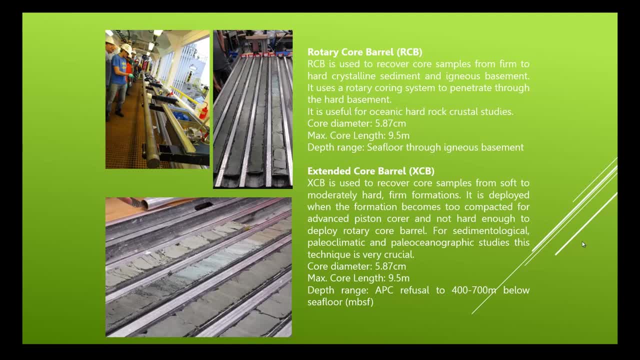 soft to moderately hard forms formations. It is used in the production of hot-treated hard rock crystals. It is used for curing of hard rock crystals deployed when the formation becomes too compact for advanced piston corer and not hard enough to deploy a rotary core bed For sedimentological, paleoclimatic and. 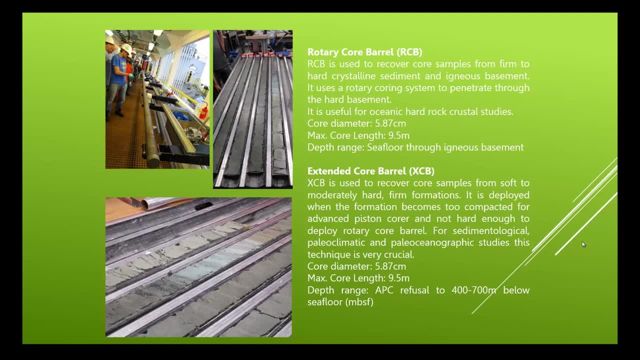 paleoceanography studies. these coring techniques are very crucial Here. the core comes with a maximum length of 9.5 meter with a diameter of 5.87 centimeter. The depth range for this coring technique is from ABC refusal to 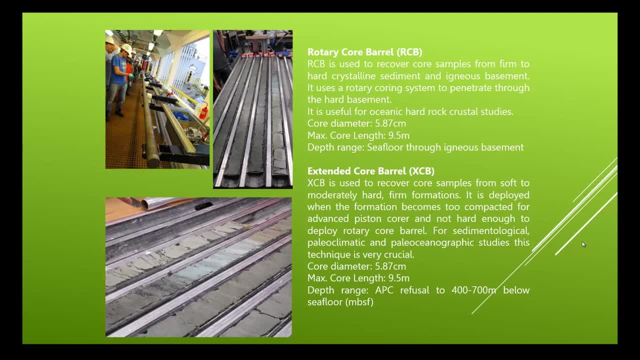 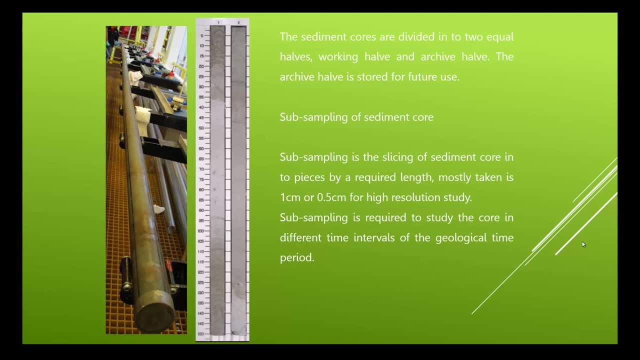 400 to 700 meter below sea floor. Now, once the core is recovered, the sediment cores are divided into two equal halves: the working half and the archive half. The archive half is stored for the future use. In this context, the next step is to 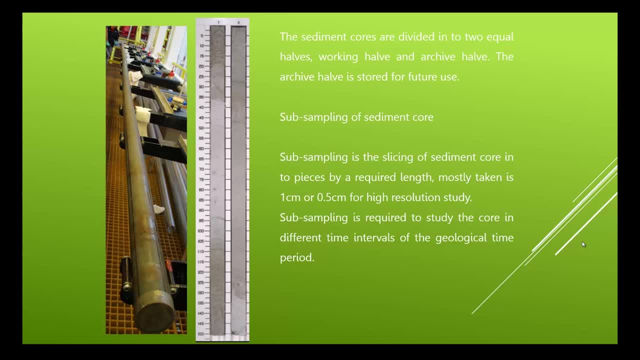 sub sample. the sediment core. Sub sampling is the slicing of sediment cores into pieces of uniform length, mostly in 1 centimeter or 0.5 centimeter. for high-resolution studies, Subsampling is required to study the sediment cores in different time intervals of the geological past. Now I'll be talking about 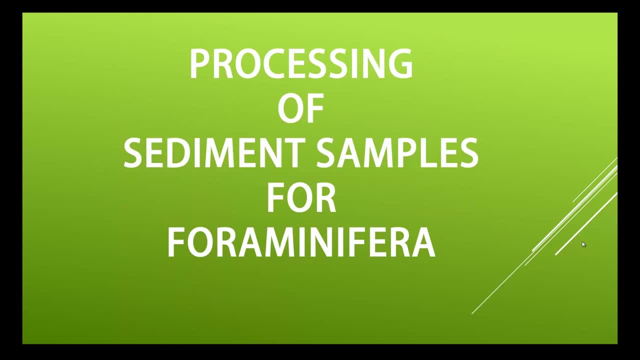 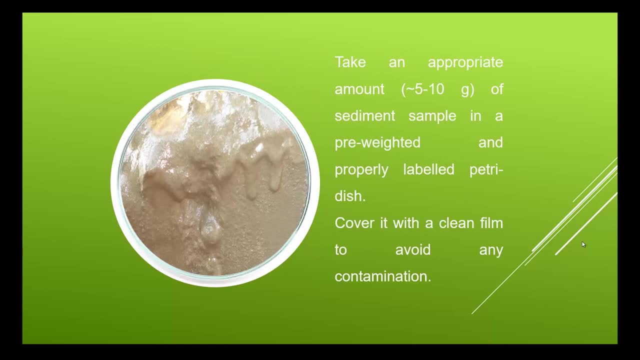 processing of marine sediment samples. for foramenifers For the processing of marine sediment samples, take an appropriate amount- nearly 5 to 10 grams of sediment samples- in a pre-wetted and properly leveled petri dish. Then cover it with a clean film to avoid any contamination. Now keep the covered. 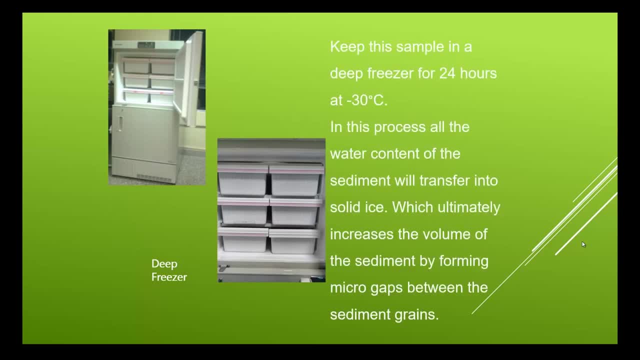 sample in a deep freezer for 24 hours at minus 30 degrees Celsius. In this process, all the water content of the sediment will transfer into solid ice, which ultimately increased the volume of the sediment by forming micro gaps between the sediment grids. Once it is completely frozen, immediately transfer the frozen 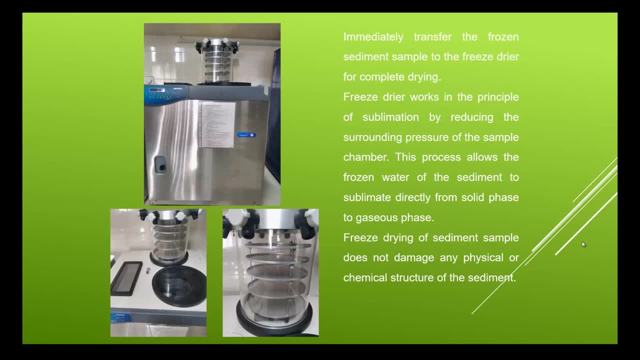 sediment samples to the freeze dryer: complete dry Freeze dryer works in the principle of sublimation by reducing the surrounding pressure of the sample chamber. This process allows the frozen water of the sediment to sublimate directly from solid phase to gaseous. 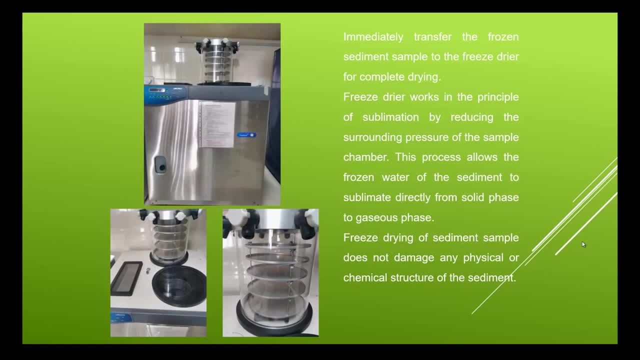 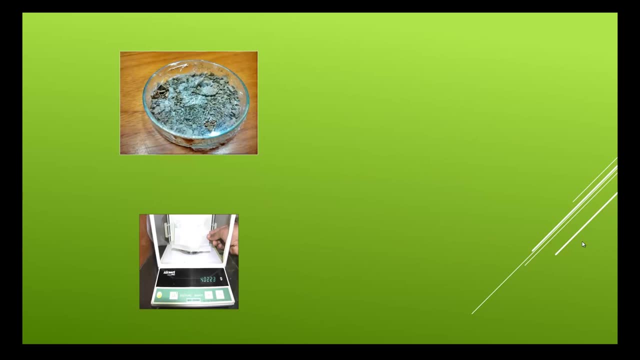 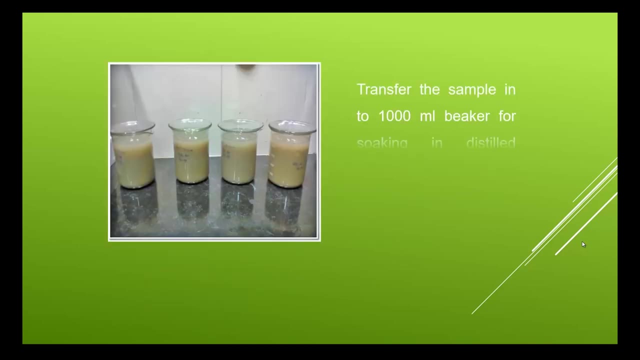 phase. In this way, freeze drying of sediment samples does not damage any physical or chemical structure of the sediment. Now, when the sample is completely dried, remove the cling film and take the weight of the sample along with the petri dish. Then transfer the sample into 1000 ml beaker for soaking in.